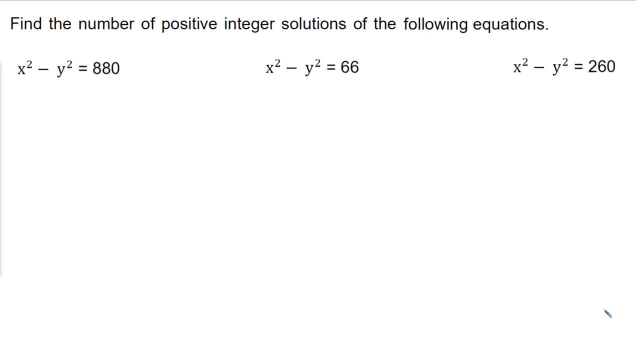 Hello everyone. in this video we are going to have a look at special equations in which x square minus y square is equal to some even number is there. In the previous video we saw x square minus y square is equal to odd number. now x square minus y square is equal to even number. The question is: find number of positive integral solutions. So there are three questions. First of all, we will do first one. First one we will do: x square minus y square is equal to 8 even number. 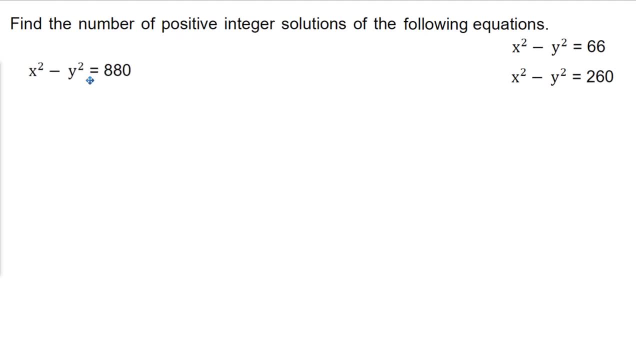 Okay, everyone. so first of all, what we are going to do is let's prime factorize. Sorry, let's do factorization. Okay, so x square minus y square is equal to what? x minus y into? x plus y is equal to 880.. Okay, so, over here. both numbers, x and y, has to be positive numbers, means they are supposed to be greater than zero. Okay, everyone. so over here, the multiplication of two numbers. the multiplication of two numbers is how much? 880.. Okay, it means what tell me out of? 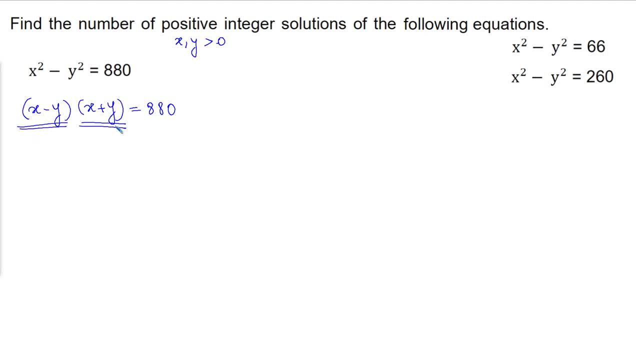 these two numbers means, out of these two brackets, at least one bracket has to be even. Okay, at least one bracket has to be even. If I consider, if I consider x minus y is even, Okay. if I say x minus y is a even number, Okay. so x plus y is going to be which kind of number? Let's see. If I say x minus y is equal to even number, Okay, everyone. So it is possible when x is odd and y is odd, Okay. or it is possible when x is even and y is even. Now let's 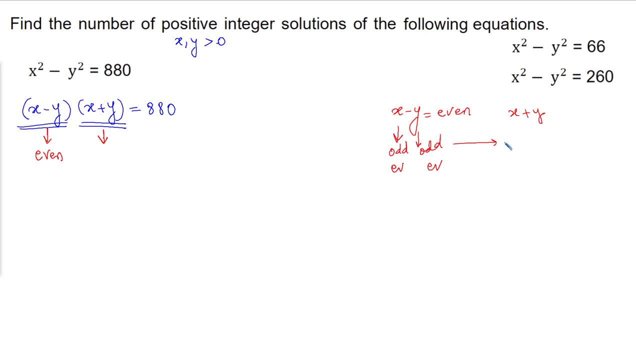 check: x plus y is how much. Okay, if both are odd number, then x plus y is going to be how much You are plus, or that is even Okay. if both are even number, then x plus y is going to be how much. 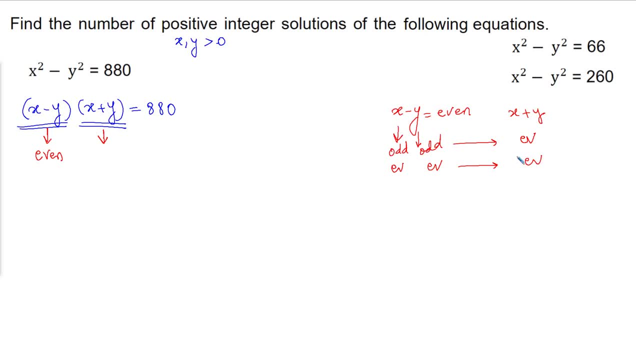 even plus even is even Okay. so if I consider x minus y is even, x plus y has to be even, only Okay everyone. Now let's do vice versa. Now, if I consider x plus y is even Okay. 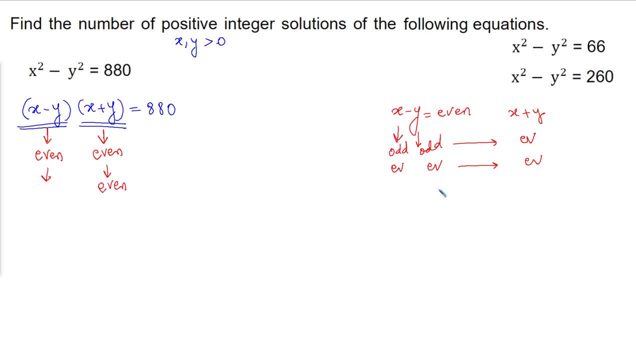 if I consider x plus y is even, x minus y is going to be what? Okay. if I say x plus y is equal to even number, Okay, that is possible. when x is odd and y is odd, Okay. or x is even and y is even, then, and then only x plus y is even, Okay. 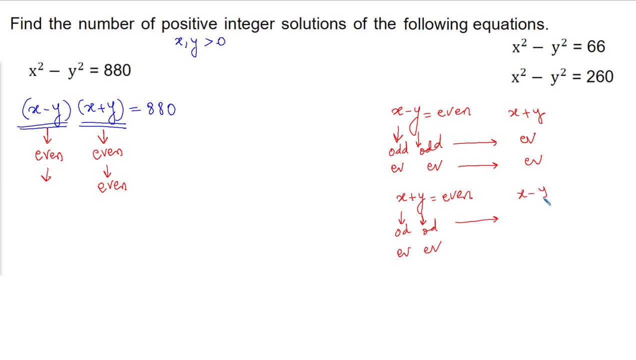 so in this case let's see: x minus y is a which kind of number? even number or odd number, Okay. odd minus odd is even. even minus even is even Okay. so if I take x plus y is even number, Okay. if I take x plus y is even number, then x minus y has to be even number only. 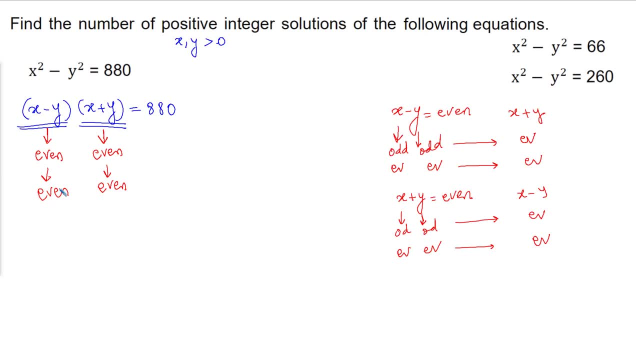 Okay, everyone. So from this, what we can conclude is: x minus y into: x plus y is equal to 880, means x minus y and x plus y. these both numbers are supposed to be even numbers. I hope everyone understood this, Okay, so what I will do is I will delete this calculation. Okay, look here. 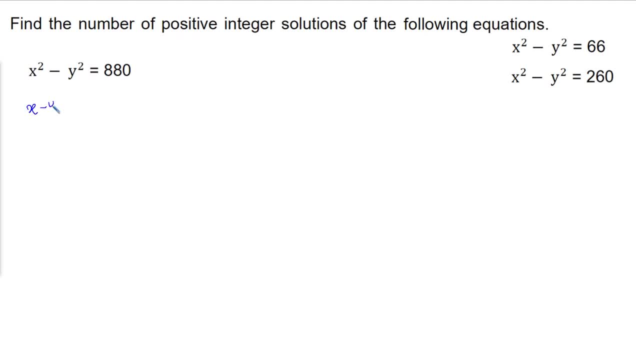 So now the first step is what tell me? first step is x minus y into x plus y. Okay, is equal to 880.. As I explained you, the multiplication of these two bracket is even, means both brackets are supposed to be even, only Okay if the x minus y is even at least one. 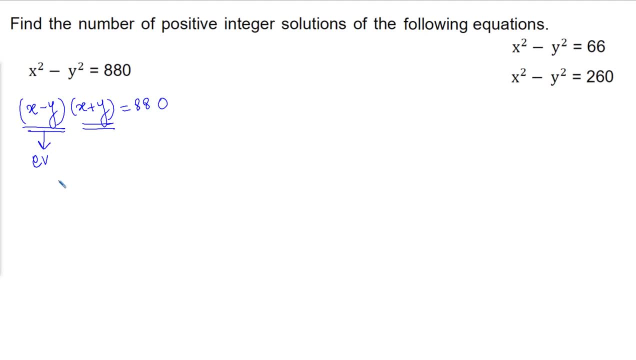 bracket has to be one. Okay, at least one bracket out of these two. bracket has to be even. But if x minus y is even, then automatically x plus y becomes even Okay. or if x plus y is even, then automatically x minus y is even. So effectively, both brackets are supposed to be even, Okay. 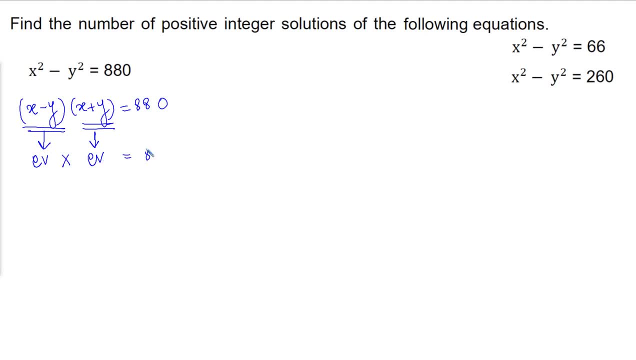 so the multiplication of these two even numbers is at 880.. Okay, the even numbers are in which format even numbers are? in a format of two into something. Okay, so let's say the value of x minus y as 2 into a and the value of x plus y as 2 into b. Okay, everyone. So 2 into a, into 2. 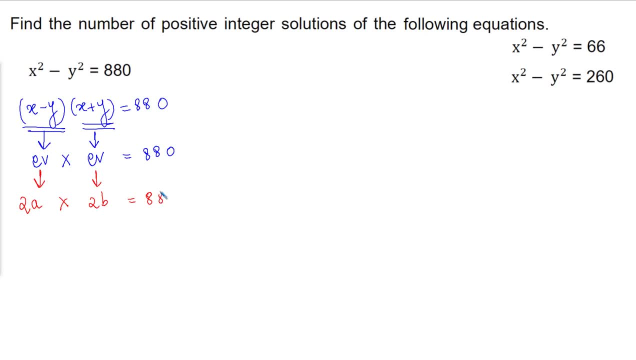 into b is going to be how much? 880.. Now, a and b can be any kind of number. Okay, a and b can be any kind of number, because if we multiply a and b with 2, it will be multiple of 2. it will be even. 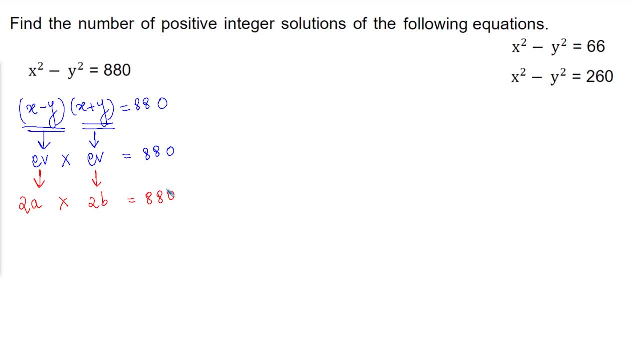 Okay. so a and b can be any kind of number- Okay, it can be even number, it can be odd number- Okay, but it has to be positive number. Okay, over here, x and y are supposed to be positive number and b are supposed to be positive number only. Okay, everyone. So over here, a into b is going. 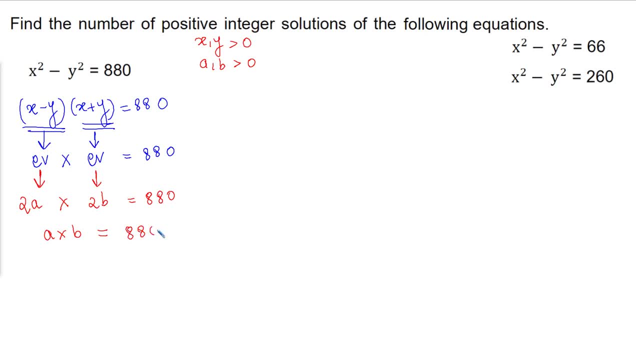 to be how much a into b is going to be how much 880 divided by 4.. Okay, everyone, 880 divided by 4, that is how much 8 into a into b- is going to be how much 220.. Done, everyone? Okay, so likewise. 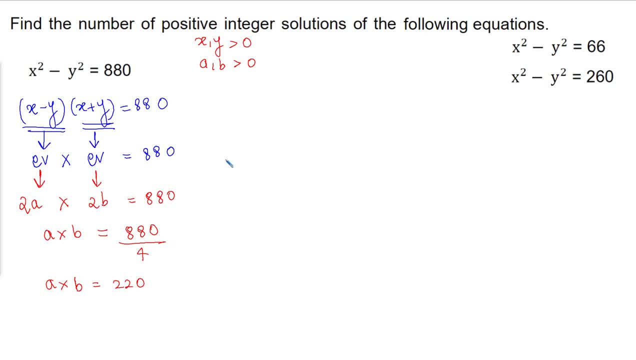 we can solve till this. Okay, Now, after this, look at, can I see? over here we consider that, over here we consider that x minus y is equal to 2a. Okay, x plus y is equal to 2b. Okay, we know that x and y are positive numbers. Okay, so subtraction of 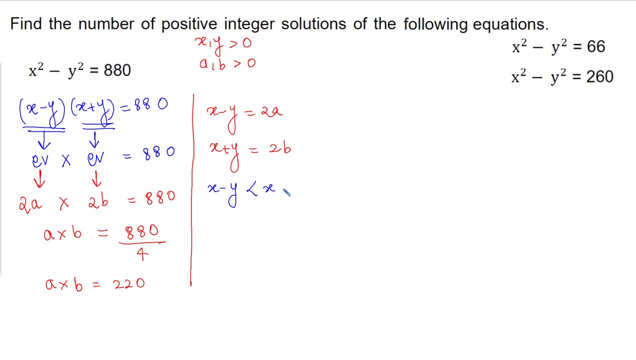 positive numbers is always less than addition of positive numbers. Okay, everyone. So from this we can see that the 2a has to be less than 2b means a has to be less than b. Okay, a has to be less than b. Okay. so 220. we can express it as what? tell me 220? we can express it as 1 into 220. Okay. 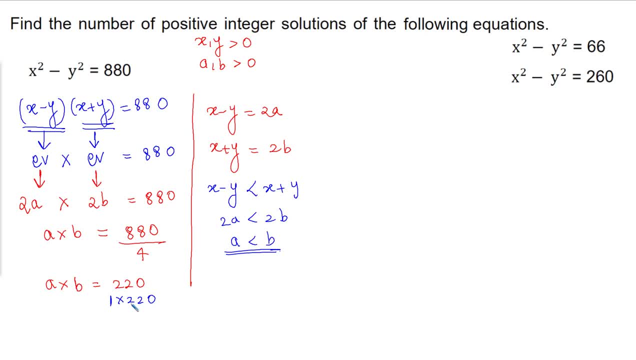 everyone. smaller number goes to a and the larger number goes to b. then we can express it as: 2 into 110.. It is not divisible by three. Okay, four into 55. And so on. Okay, we can list it down. Or what we can do is: the prime factorization of 220 is how much? Okay, 220 is equal to how much. 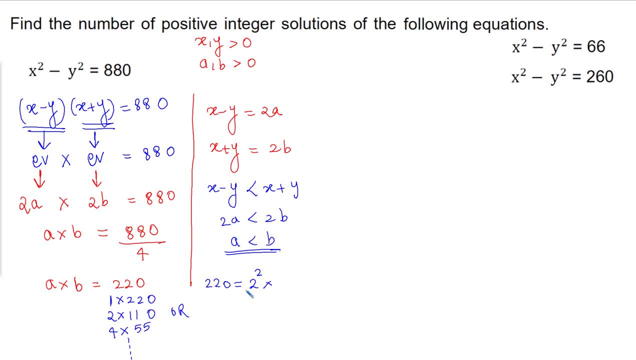 two square, two square into 55.. Okay, 55 into four. Okay, that is two square into five to the power one, into 11 to the power one. So over here the number of factors are going to be how much Two. 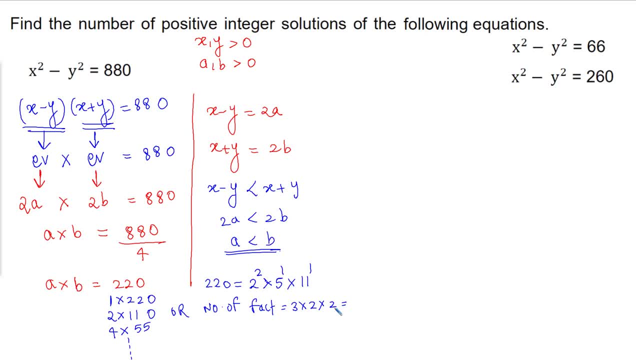 into one plus one is two into one plus one is to that number of factors are going to be 12.. Okay, everyone. So in how many ways? in how many ways we can express it as a product of two numbers, in one by two into 12.. That is total. there are six ways Total. there are six ways we can express it into. 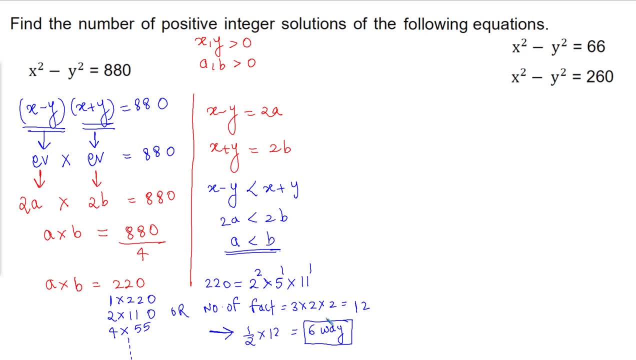 the product of two numbers, Okay, everyone. So a into b is equal to 220.. In how many ways we can express: a into b is equal to 220, in total six ways. So every way will give us only one solution, Okay. 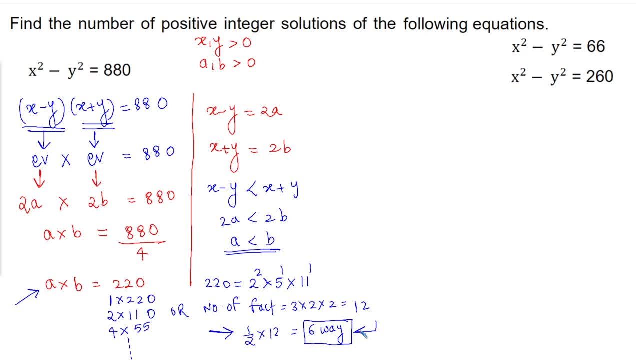 we cannot do us one into 220. We cannot write 220 into one, because smaller number should go to a and larger number should go to be okay. One into 120. Sorry, one into 220. We cannot write it as minus one into minus 220. Or we cannot write it as minus 220 into minus one, because sum of two positive. 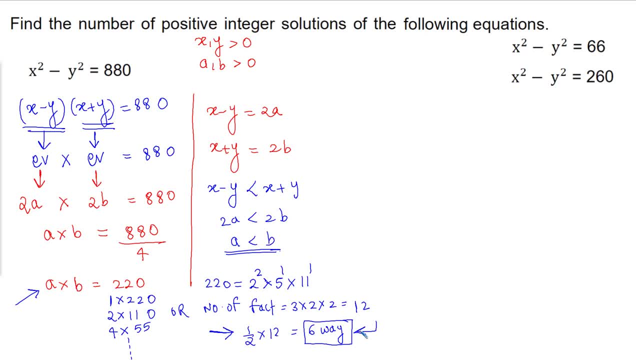 numbers has to be positive number only, Okay. So every way will give us only one solution. So, over your two, over here, total, how many solutions are going to be there? Total, six solutions are going to be there. So answer is: six positive integral solutions. Okay, everyone Likewise. 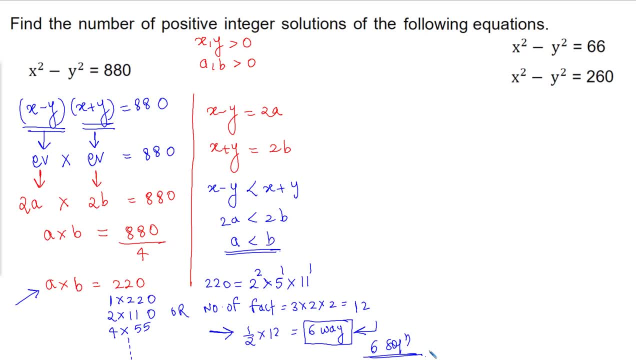 we can solve this. Okay, So over here there is one small. there is one small observation. Okay, there is one small observation. Okay, So over here, this number, over here, look at this number: 880.. Okay, this number, 880, should be divisible by four. Okay, Because at this state we are going. 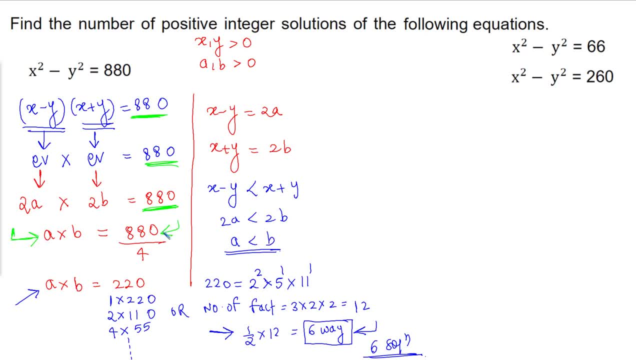 to divide 880 by four. Okay, If 880 is divisible by four, if that number is divisible by four completely, then and then only we can solve this. Or you can say that then and then and then and then only it is going to have at least one positive integral solutions. Are you getting this? 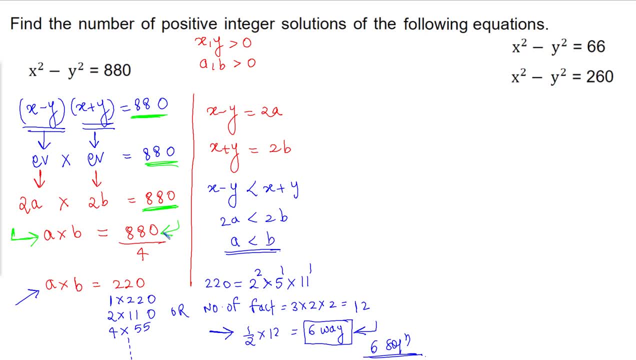 Okay, So if this 880 is over here, 880 is luckily divisible by four, so that we can proceed If 880 instead of 880, if there is some another number which is not divisible by four, then the answer is going to be: how much? The answer is going to be zero solution because a and b are integers. 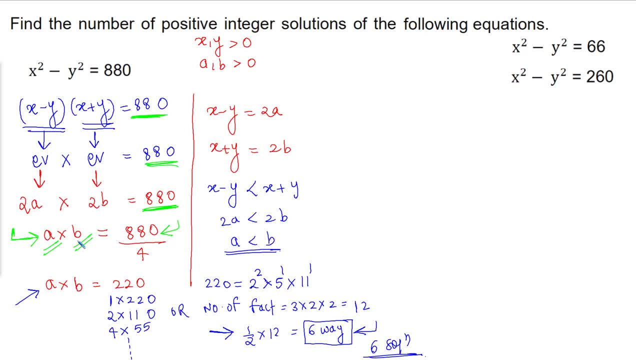 a and b are positive integers, Okay. The product of positive integers is going to be integer only, positive integer only. It cannot be fraction, It cannot be decimal number, Okay. What I'm saying is: the product of integers is always integer, Okay. It cannot be fraction, It cannot be decimal, Okay. So over here, x square minus y. 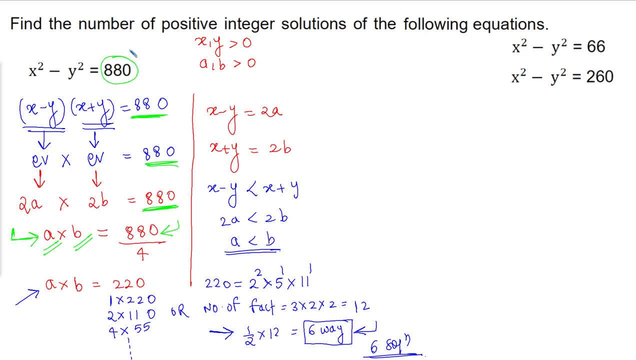 square is equal to. if this is a even number, then this number has to be multiple of four. Then, and then only, we will be getting integral solutions. If this number is not, if this number is even and not a multiple of four, for example, 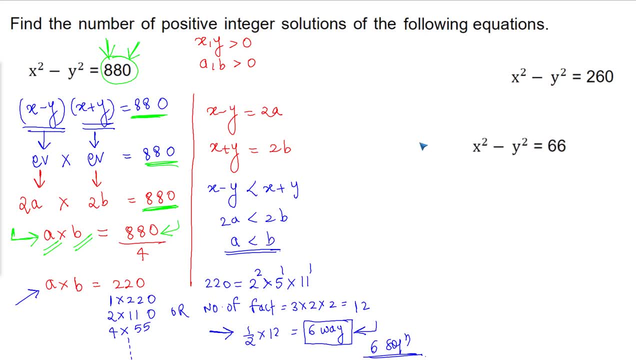 look at: x square minus y square is equal to 66. okay, this number is even. This number is even, but this number is not a multiple of four. This number is even, but not a multiple of four. okay, everyone. So at this state we will get stuck here. Okay, so 66 is not divisible by four. the product of two. 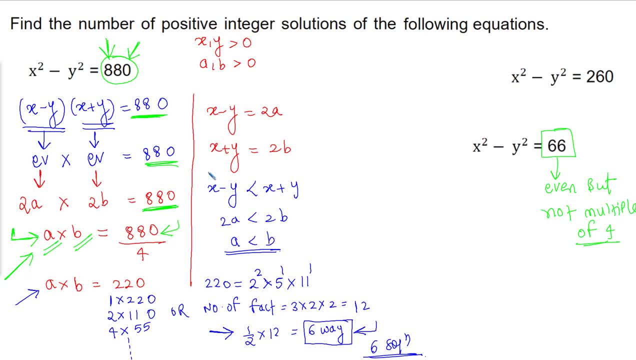 integers cannot be a fraction. okay. so for this question, the answer is going to be how much? the answer is going to be zero. zero positive integral solutions, okay, everyone. zero positive integral solutions, okay. so what we need to remember is if x square minus y square is equal to even number, and if that even number 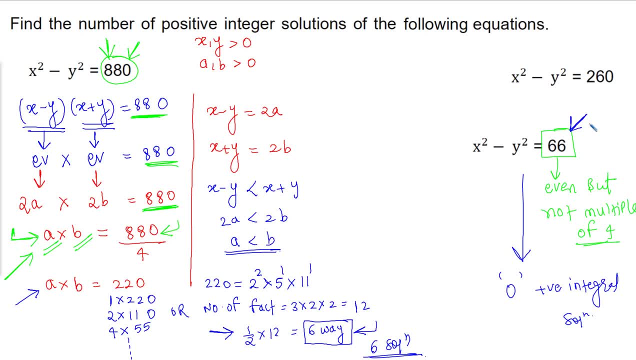 is not a multiple of four, then answer is going to be zero integral solutions. okay. so what we need to remember is: if x square minus y square is equal to even number and that number has to be multiple of four, then, and then only, we will be getting integral solutions, okay, everyone. 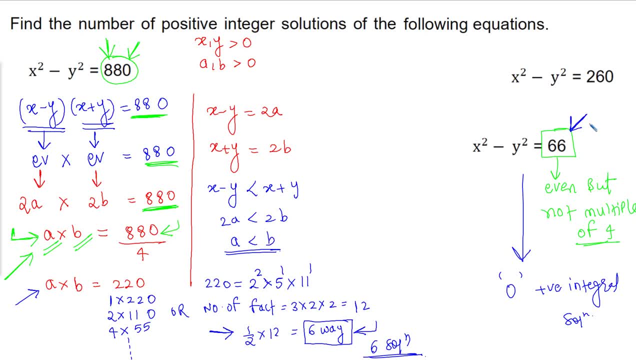 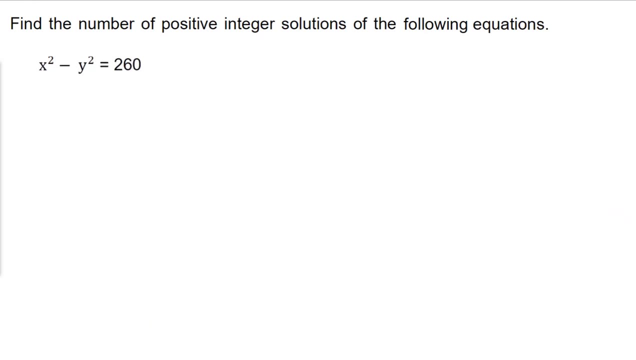 i hope everyone understood this. okay, now let's do one more: x square minus y square is equal to 260. okay, so now i hope everyone understood this so we can be. we will be able to do this quickly. now look at the question: is x square minus y square is equal to 260? okay, everyone. the first. 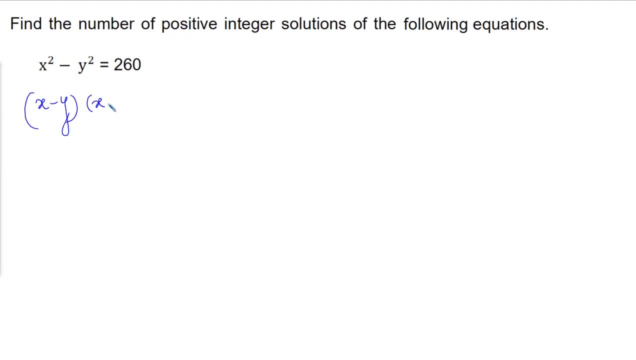 step is what x minus y into? x plus y is equal to 260. okay, the product of these two bracket is even. number means at least one of the bracket has to be even. so if first bracket is even, then automatically second bracket also becomes c1. okay, so the first bracket is even. it should be in a. 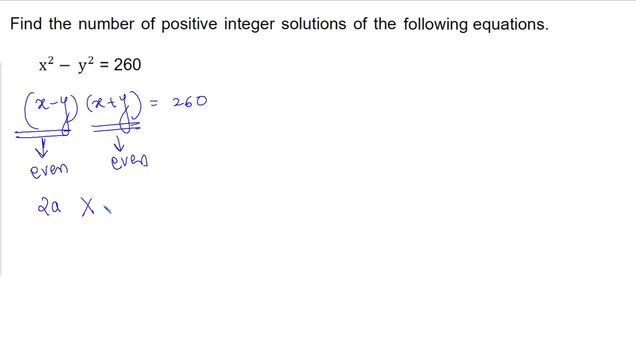 format of 2 into a second bracket is also even it should be in a format of 2 into b is equal to 260. so over here the value of a into b is going to be how much 260 divided by 4. so the value of a into 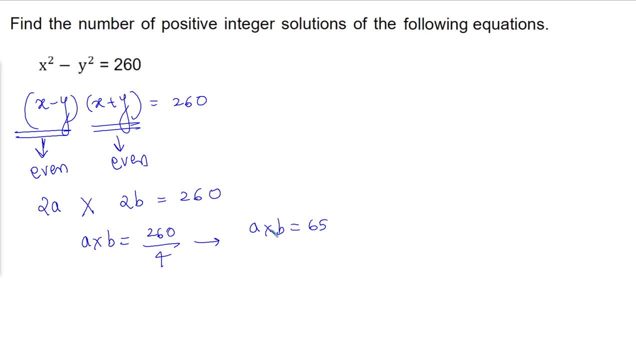 b is going to be how much? 65? okay, everyone. so now over here. x and y are positive okay. so now over here. x and y are positive integers, okay everyone. so a and b are also positive integers, okay. so the subtraction of two positive integers is always less than the addition of two positive integers. so value of 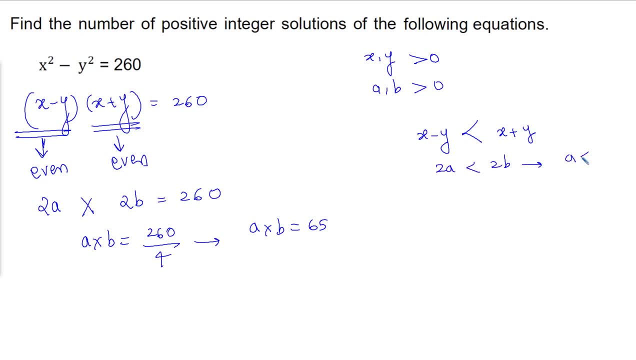 2a should be less than 2b means a should be less than b. okay, everyone. so 65. we can express it as 1 into 65. okay, then 5 into 13. these are the only two ways, okay, these are the only two ways in which. 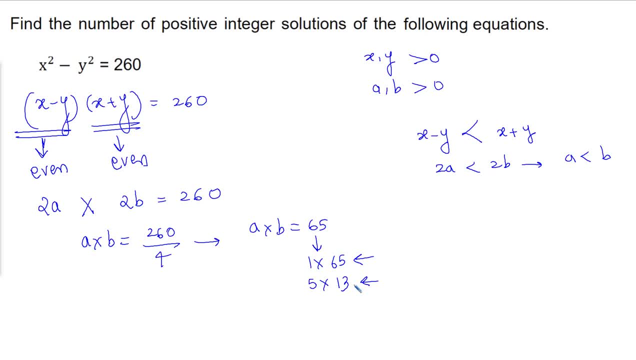 we can express 65, okay, so smaller number in every pair, smaller number goes to a and larger number goes to b, okay, everyone. and we cannot reverse. we cannot reverse because smaller number goes to a only okay and the larger number goes to b. we cannot take negative possibilities because sum 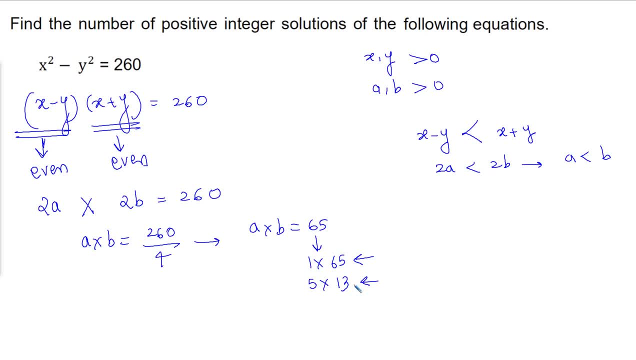 of two positive integers cannot be negative number. okay, so over here, the answer is going to be: how much answer is going to be? there are two ways. every way will give us one, one solution. okay, so total: how many solutions will be there? total: there are two positive integral solutions. are there two positive integral solutions? are there?